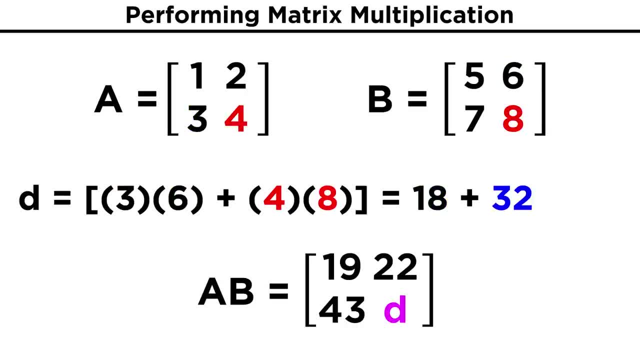 Three times six is eighteen. Four times eight is thirty-two. Eighteen plus thirty-two is thirty-two. Four times six is eighteen. Four times seven is fifty, and that will go in the last entry here. This is the algorithm we will follow for matrix multiplication. 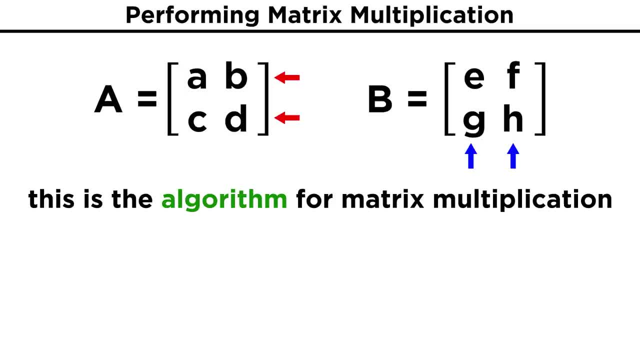 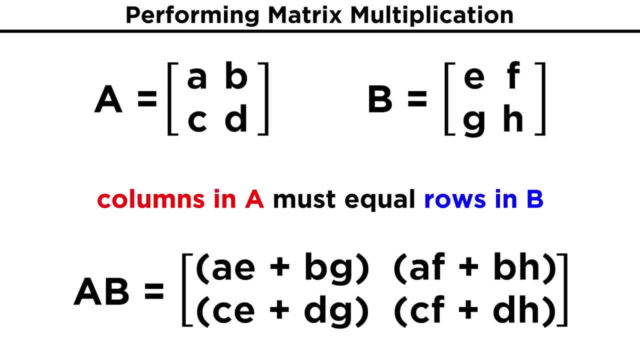 We are using rows from the first matrix and columns from the second matrix and we are finding the sum of the products of the corresponding entries. This explains why the first matrix has to have the same number of columns as the second matrix has rows. 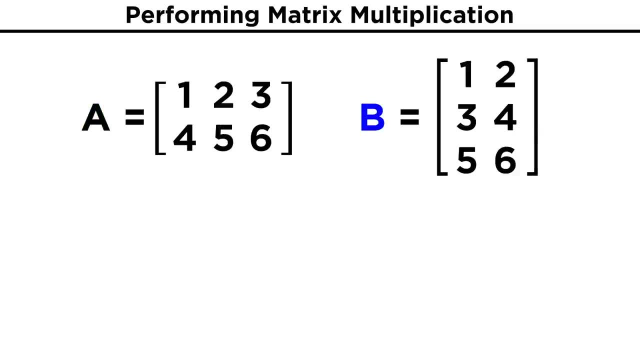 Take something like this: two by three matrix times this other three by two matrix. These can be multiplied in this order and once we begin we can see that the three entries in the first row of this one correspond to the three entries in the first column of this. 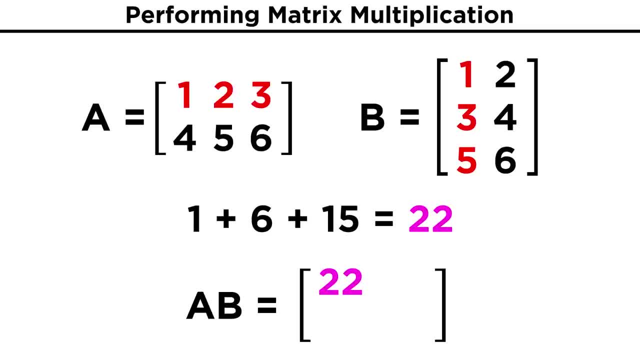 one. We add up the numbers and there is our first entry in the product matrix. Then we use the second column and then we repeat this process for the second row of the first matrix. This gives us a product matrix that is two by two. 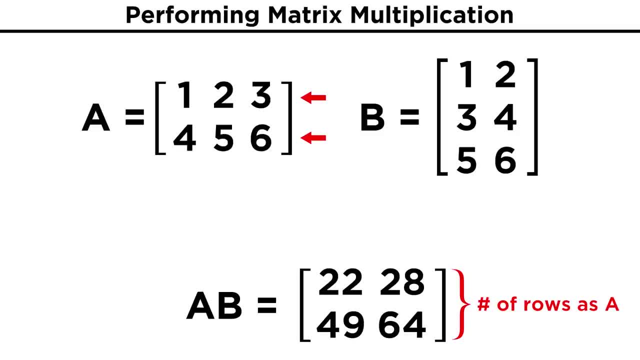 So the product matrix will always have a number of rows that is equal to the number of rows in the first matrix and a number of columns that is equal to the number of columns in the second matrix. This also tells us an important fact that may not have been immediately intuitive. 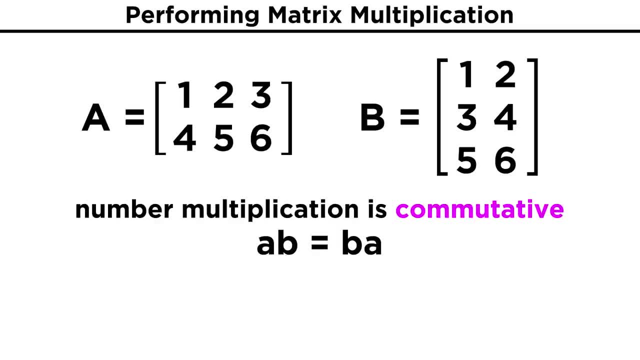 Although the multiplication of numbers is commutative, the number of rows in the first row is commutative, meaning that A times B is the same as B times A. This will not be the case for matrix multiplication. Take the two by three and three by two matrices we just multiplied together. 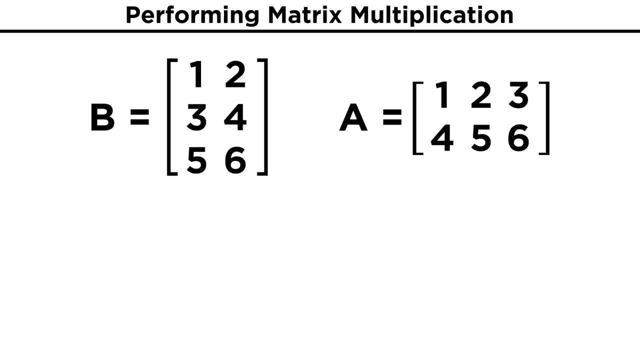 If we switch their order, we will get a completely different result: a product matrix that is three by three rather than two by two. As you can see, the three rows from the first one and the three columns from the second one will determine these dimensions. 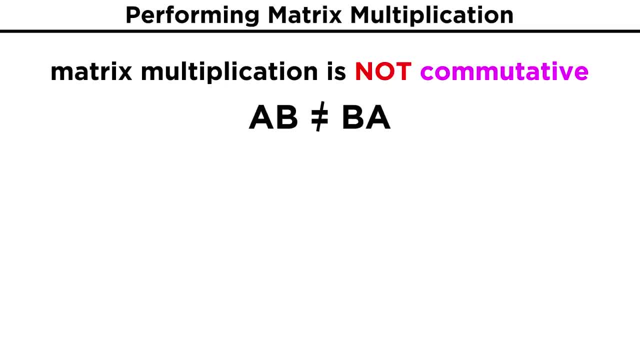 So matrix A times matrix B is not equivalent to matrix B times matrix A. However, matrix multiplication is associative, meaning that if we are multiplying three matrices in a specific order, it doesn't matter which pair we multiply first. In addition, the distributive property can apply in some cases.